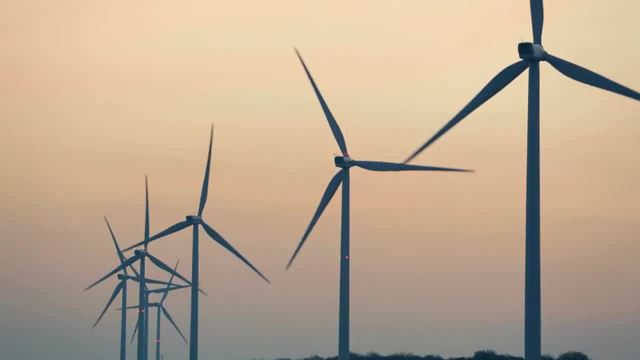 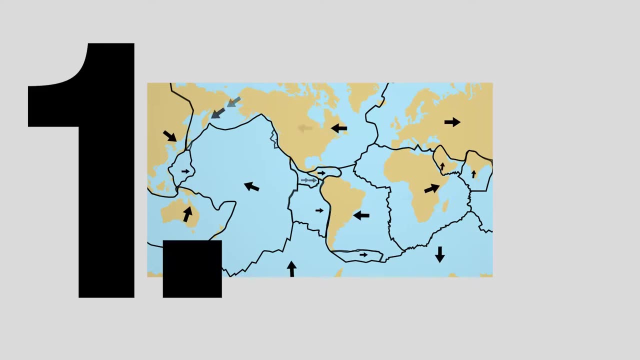 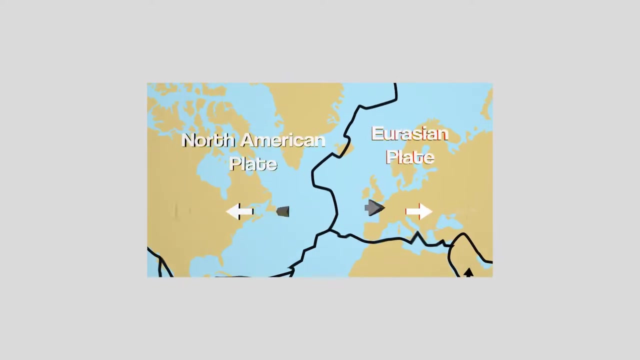 peddling on it. A wind turbine gets the energy to move from, well, the wind. As we covered in video 1.03, Earth's crust is made up of huge slabs of rock called tectonic plates, and those plates are moving. They get their energy from convection currents. 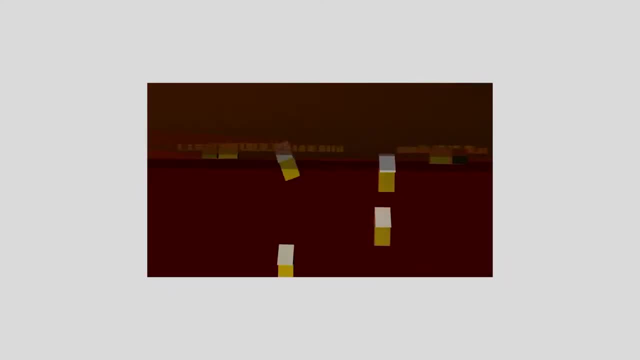 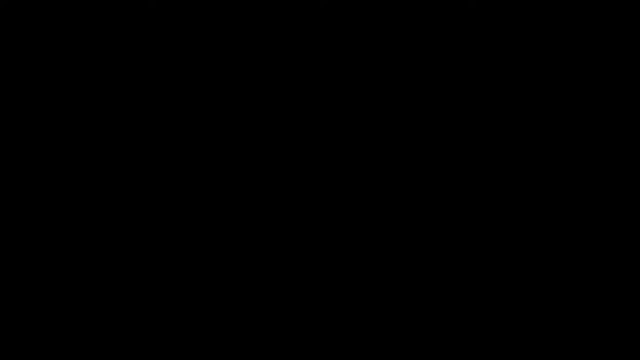 in the mantle underneath them, which keeps them moving slowly over forever. They get their energy from convection currents in the mantle underneath them, which keeps them moving slowly over forever- thousands of years, or it it would if they didn't keep getting stuck. let's show you how this works. 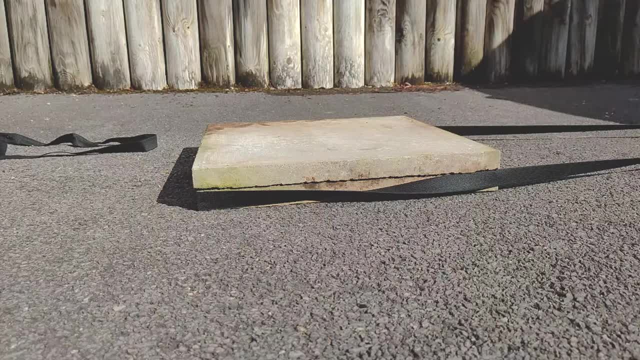 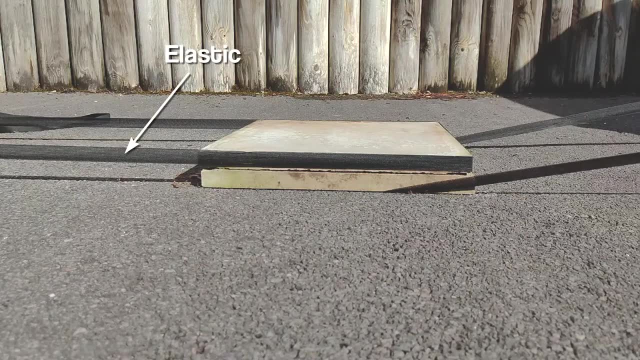 with a little experiment here. we have two paving slabs which are going to be our tectonic plates. we're going to use some elastic to make the tectonic plate on top move to the left and the one underneath move to the right, in real life, the closest thing. 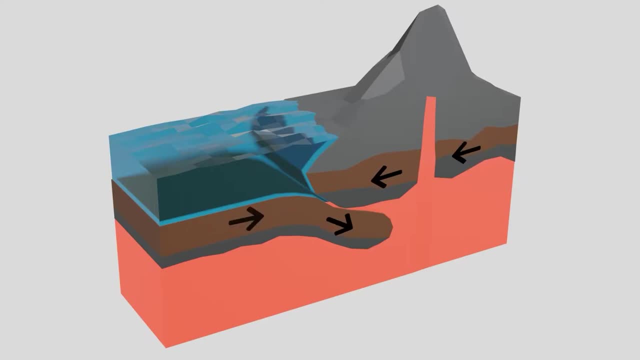 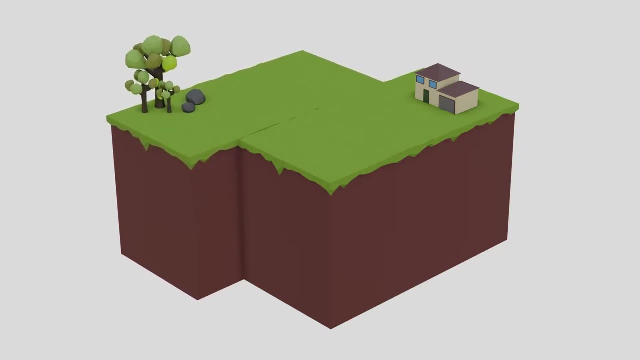 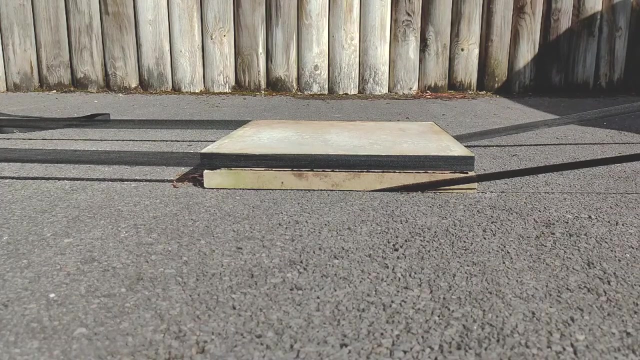 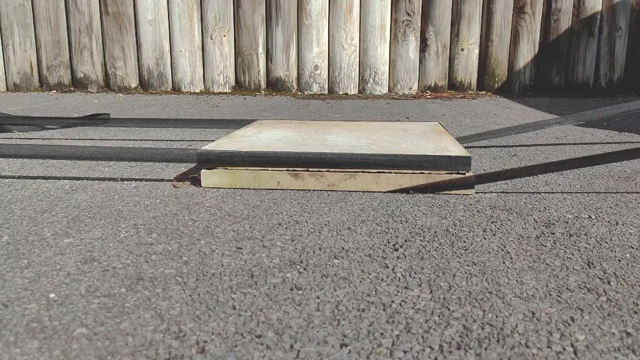 we have to. this would be a destructive, also known as convergent plate boundary, although if you imagine you were looking at this from a top-down view, it would also show a conservative or transform plate boundary. as the elastic is pulled tighter, energy continues to build up, it builds and builds until eventually so much energy has been put in that the slabs become. 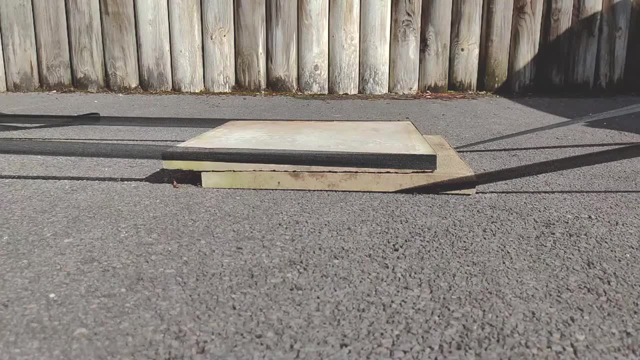 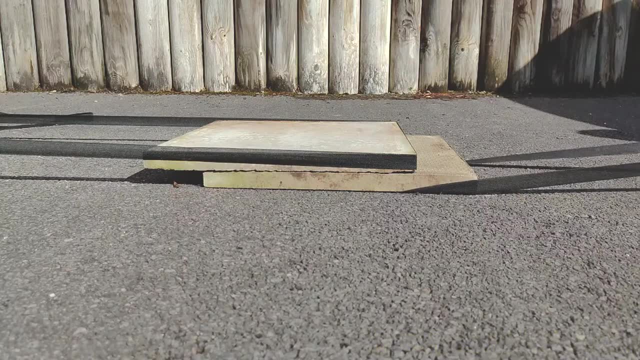 unstuck and release all of that stored up energy in one violent jolt. that sudden release of energy when the plates move is an earthquake. i'll admit that it's not a good idea to build a tectonic plate. the energy released that's released by these concrete slabs isn't very much. but imagine this. 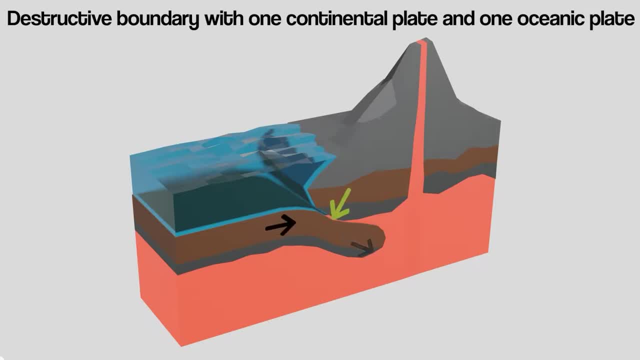 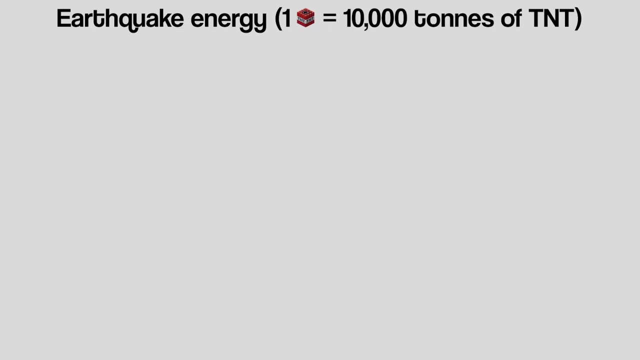 happens in between two of the earth's huge tectonic plates. when they finally build up enough energy to jolt into motion, it can release a colossal amount of energy. you can't even begin to imagine how much energy a strong earthquake releases, but to try and give you some kind of idea. 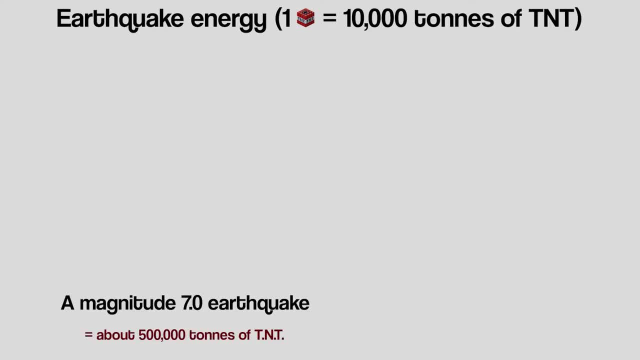 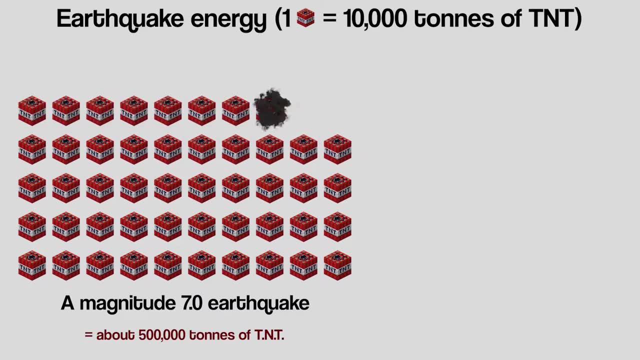 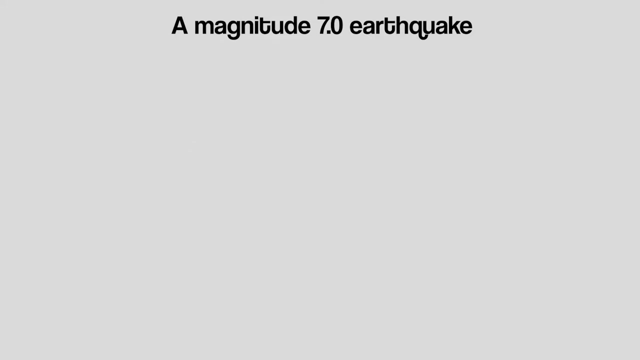 a magnitude 7 earthquake releases about the same amount of energy as 500,000 fans per second thousand tons of TNT exploding. For comparison, the nuclear bomb that was dropped on Hiroshima during World War two released an amount of energy similar to just 15,000 tons of TNT. This means a magnitude 7 earthquake releases the same. 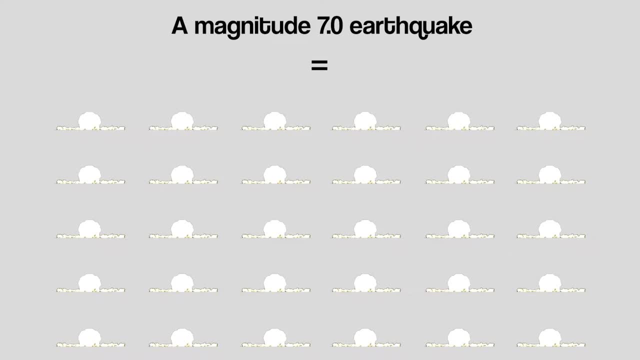 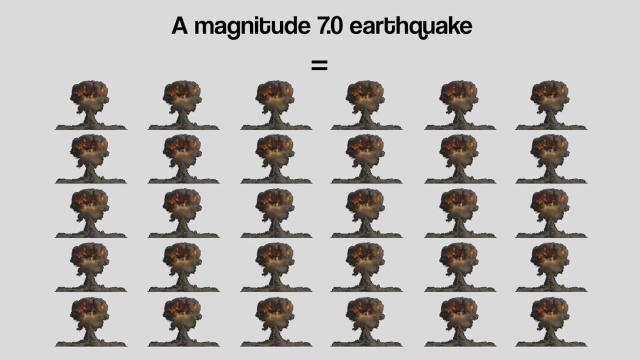 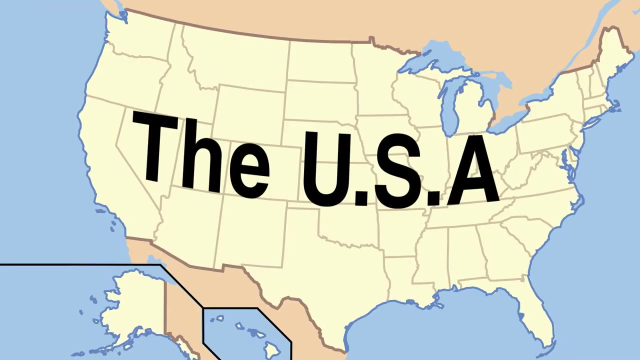 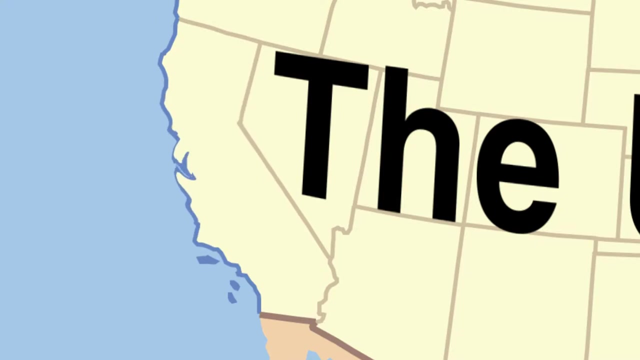 amount of energy as 30 nuclear bombs going off at once. And, as you'll see in our next video, earthquakes get much, much more powerful than magnitude 7.. So when the earthquake happens and all that stored up energy is released, what comes next? Well, the short answer is waves. Energy likes to travel in waves. 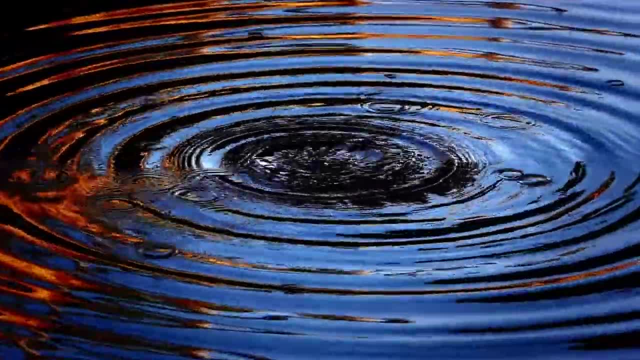 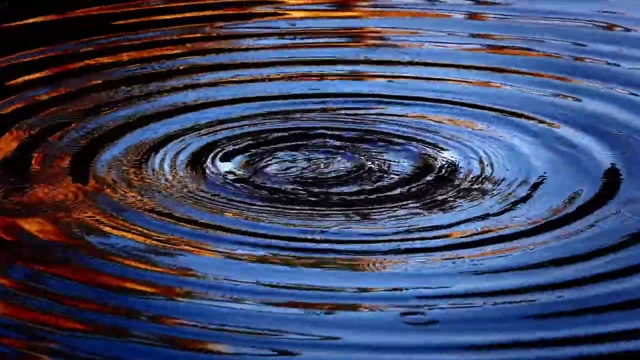 When you throw a stone into a pond, you are transferring the energy of that stone into the water And it sends small waves of energy through the water, which we know as ripples. This might be a little weird when you first hear it, but if you put 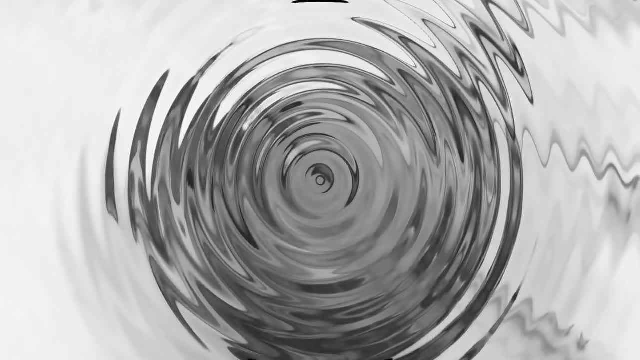 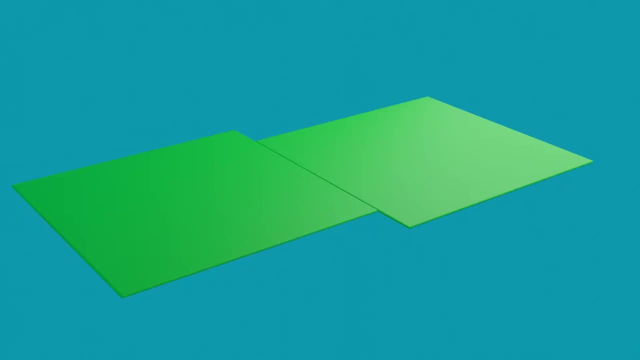 enough energy into it, the ground can ripple just like water. That energy, of course, comes from the earthquake. Here is a simulation we made to show you what's going on. When the tectonic plates suddenly become unstuck and the earthquake begins, all the stored up energy is released into the ground as it. 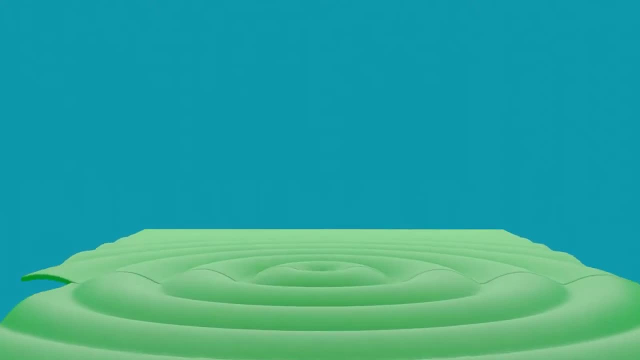 spreads outwards just like ripples in a pond. Once we open up the path, we typically see the COM libraries that you have to такого happened a bit over this. If we cut the ground open to show you the exact point where the earthquake is, 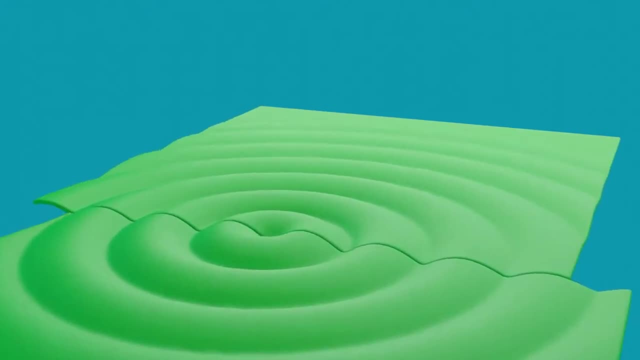 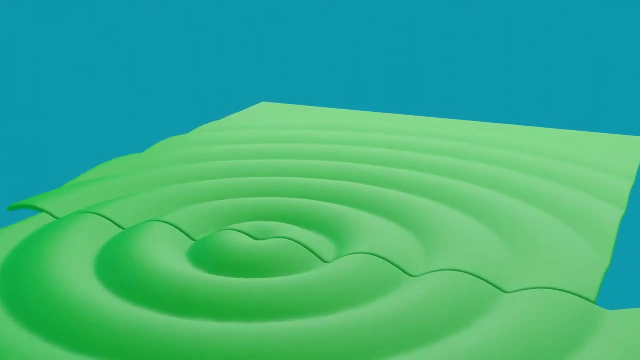 starting. you can see how it's all: just waves traveling through the ground. Oh, and there's a name for the starting point of the earthquake, by the way, but we'll come back to that in a moment. It's these huge waves of energy travelling through the ground that caused the damage To us humans. these 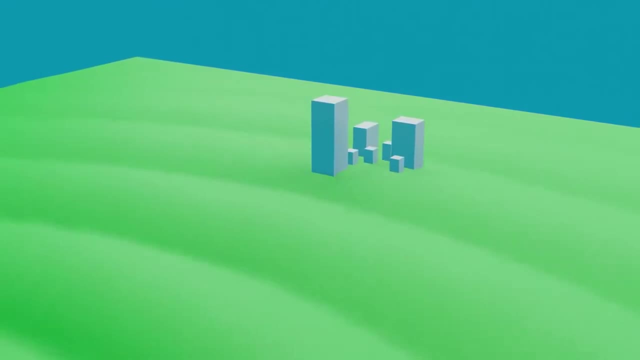 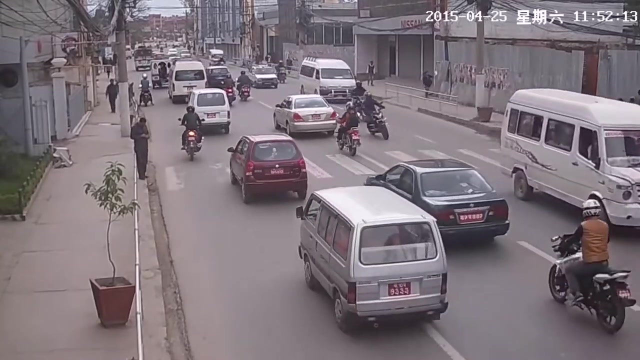 waves travelling through the ground feel like intense shaking- well not moving. When these huge waves of energy are travelling through the ground beneath them, weaker buildings can easily crumble and collapse, often injuring or killing the people inside, As crazy as that is to imagine. look at this footage from Nepal earthquake in 2015.. 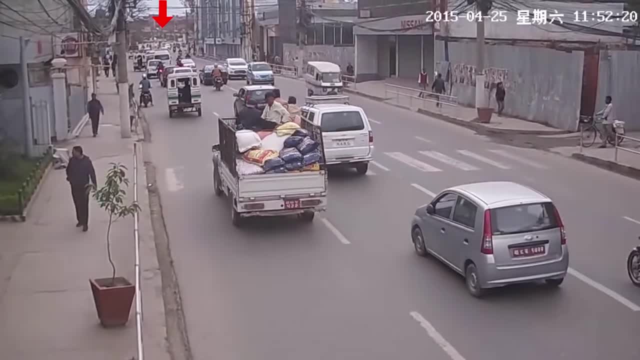 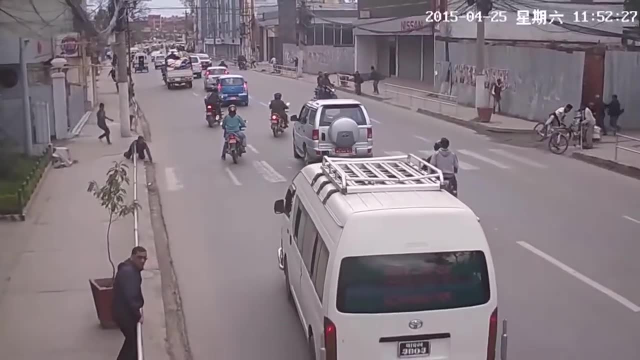 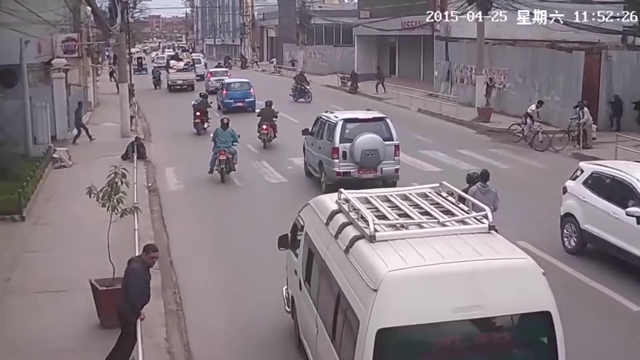 You see those buildings right at the end of the street. If you look carefully, they look like they're moving separately to what's going on closer to the camera. That's because those ripples of energy from the earthquake are travelling through the ground towards the camera. Also, if we slow this footage right down, 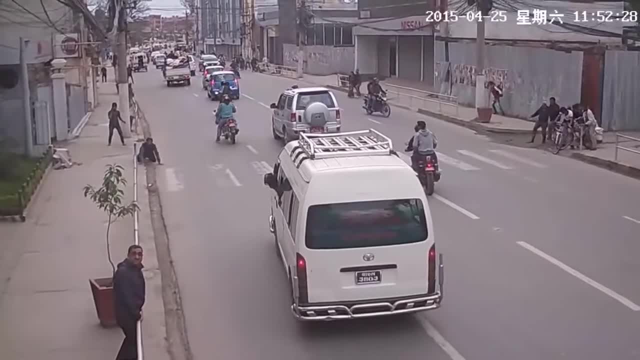 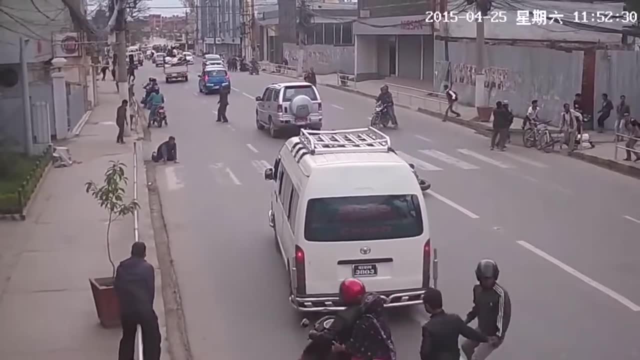 take a look at how the people are thrown off balance by the ripples moving through the ground. It's not random at all. They're being thrown side to side by the waves of energy as they pass through the ground beneath their feet. That's why an earthquake makes the ground. 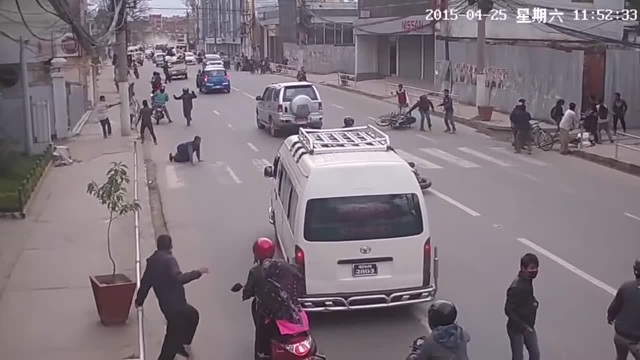 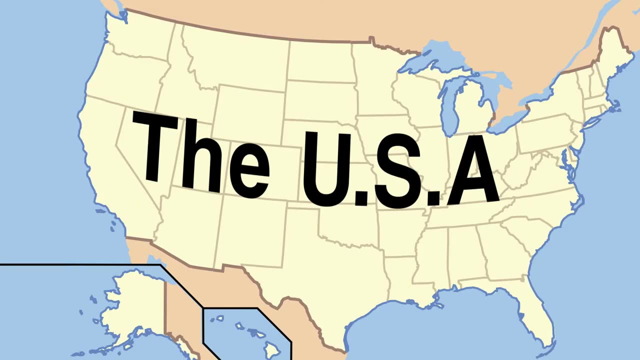 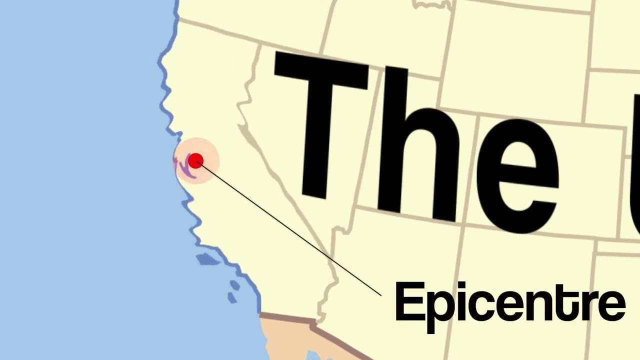 shake. All of that movement in the ground causes everything on the surface to shake violently. When an earthquake takes place, one of the key things we need to know is where it happened. We call this the epicentre of the earthquake. It literally means the point on the earth's surface. 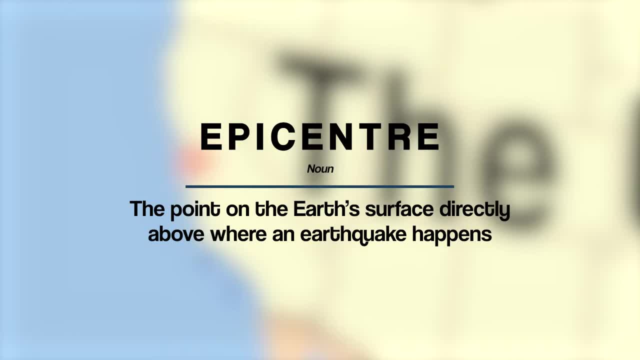 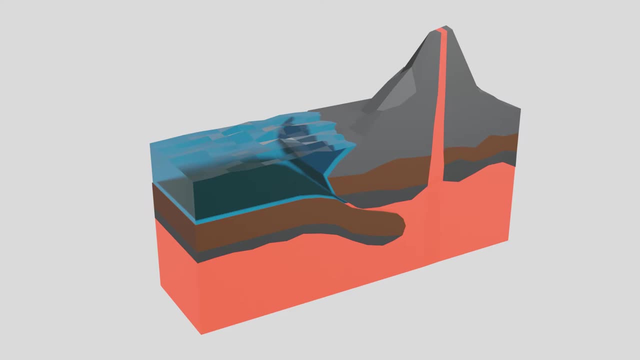 directly above where an earthquake happens, the place where the waves of energy ripple outwards from. But hold on a second. What do we mean when we say directly above where the earthquake happens? Well, as we know, earthquakes happen underground, But they don't all happen. 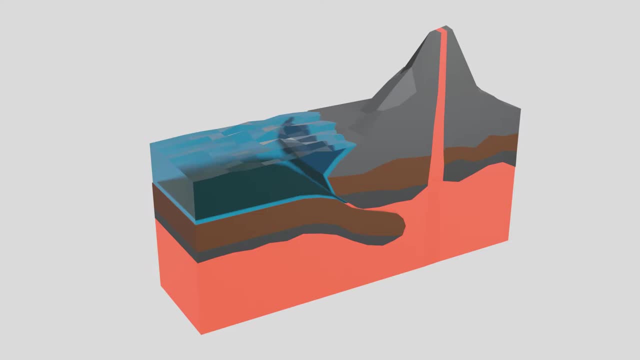 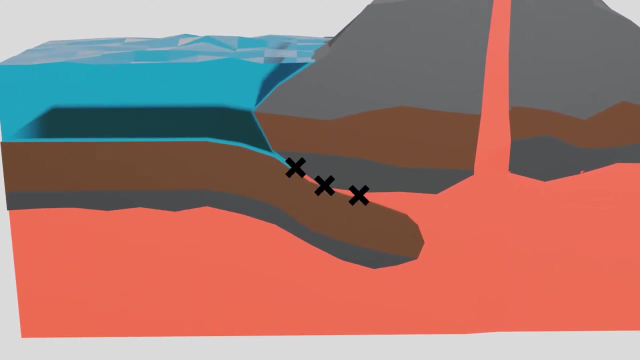 at exactly the same depth. Think about a destructive boundary like the one we've explained before. As the denser tectonic plate subducts underneath the other one, they grind together and get stuck. But they could get stuck here or here or basically. 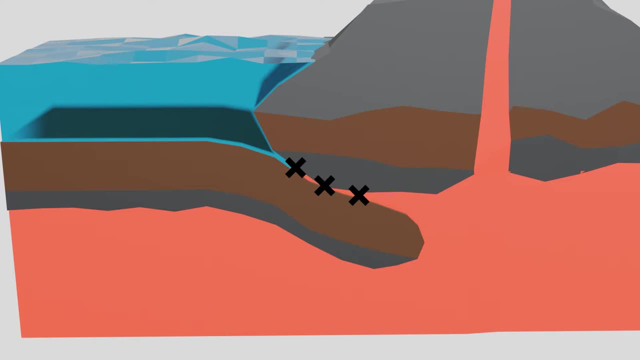 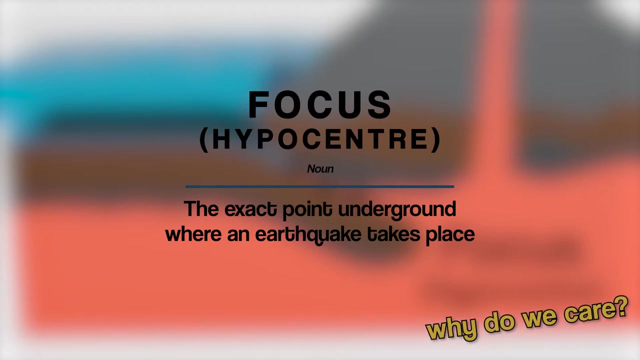 at a point where the plates are touching each other. This is where we get the term focus, the hypocentre of the earthquake. But focus works just fine. The focus means the exact height underground where an earthquake takes place. But why do we care how deep the focus? 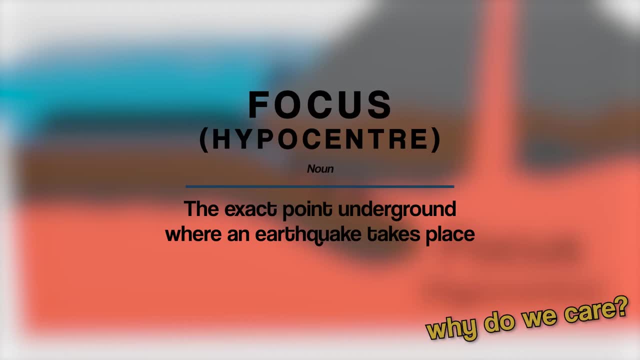 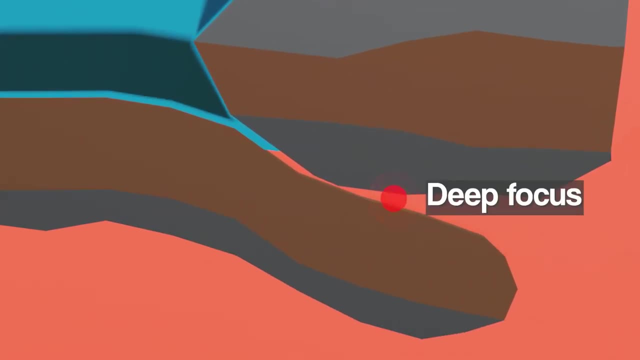 of an earthquake is Well, the answer is: it could actually make a really big difference in how destructive an earthquake is. If the earthquake has a deep focus – meaning it happens quite far underground – the energy from that earthquake spreads out a lot and weakens 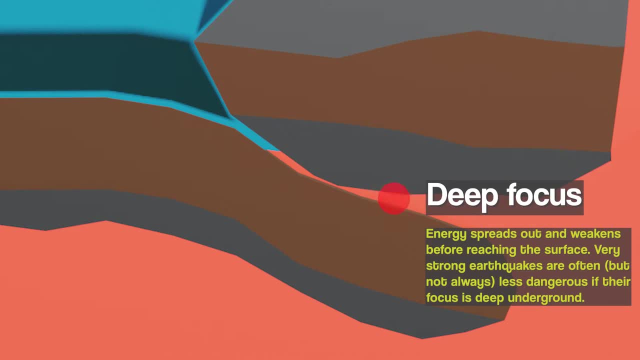 strong earthquakes end up not causing a lot of damage if they have a deep focus, As you might expect. shallow focus earthquakes are the opposite. They don't happen very far underground at all, so the concentrated energy released by the earthquake reaches the surface quickly, often causing massive destruction even if the earthquake isn't that strong.